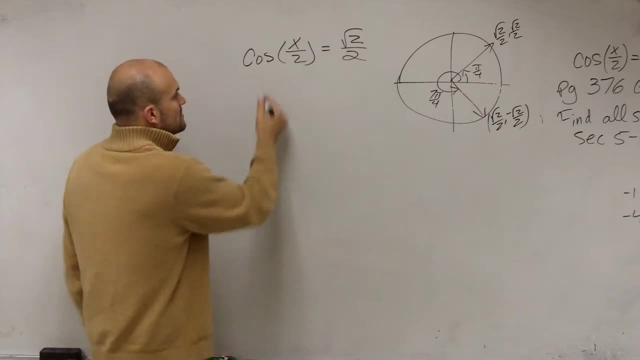 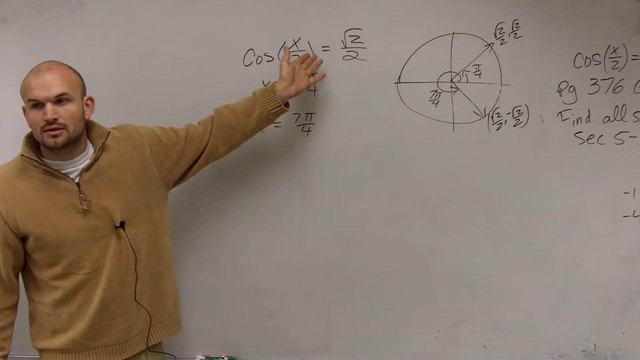 So you could write your answer. What we did before was we wrote x equals pi over 4 and x equals 7, pi over 4.. Now the difference is we're not solving for our variable, our angle, that we're taking. the angle is not just x, x, it's now x divided by 2.. 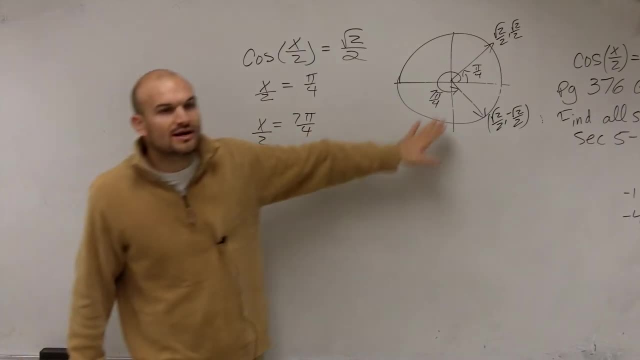 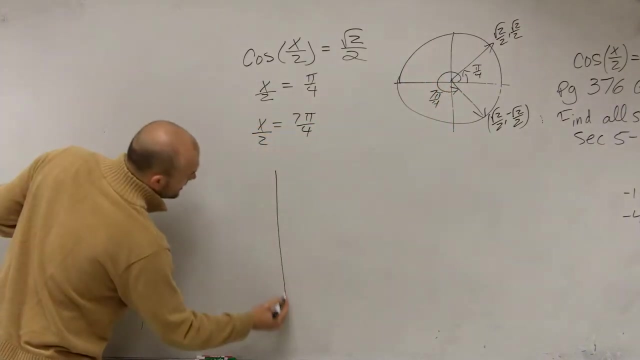 And the other issue, though, is we're not just finding the angles that are on the unit circle, That's the interval between 0 and 2 pi. I want to find all of the solutions. So to help you kind of visualize what that looks like, let's go back and draw the cosine graph again. 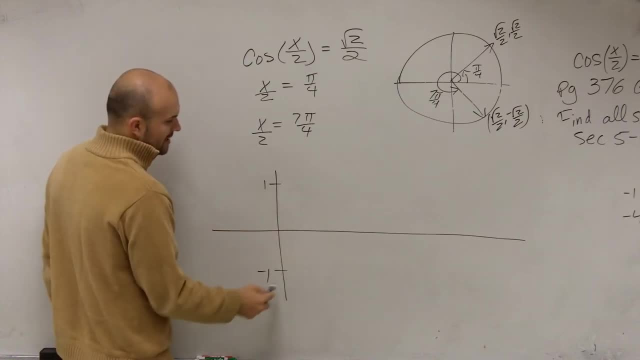 So if I was going to draw the cosine graph- we know it goes up to 1, down to negative 1.. 1,, 2, 3,, 4,, 5, 6.. Okay, 1,, 2, 3.. 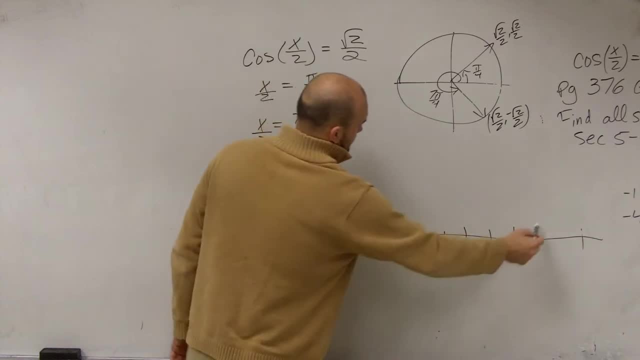 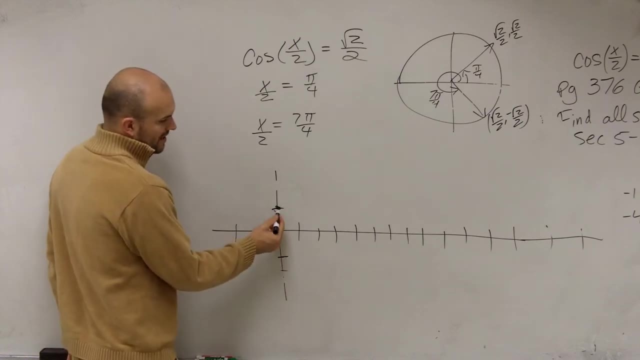 Let's actually let's make this a little bit smaller. Okay, so we know the cosine graph goes at 1, comes down minimum, comes up there. So the distance from here to here is 2 pi, right? Does everybody see this? 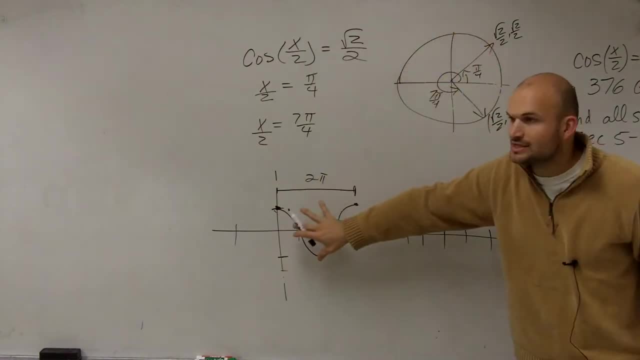 This is represented right up here. We learned how to graph it like this by using the points on the unit circle. Because this This is represented right up here. We learned how to graph it like this by using the points on the unit circle. 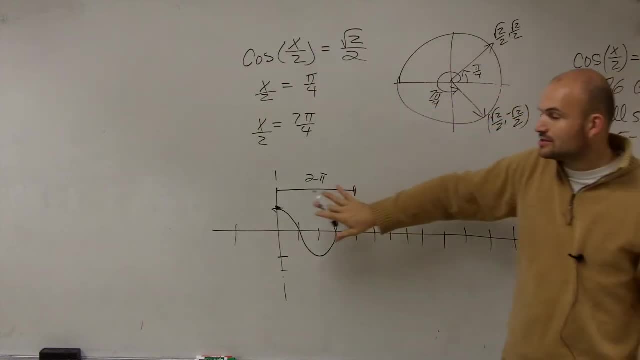 This is represented right up here. We learned how to graph it like this by using the points on the unit circle. This is an interval of angles between 0 and 2 pi. So here is what it's going to look like when we graph it on an x and y axis. 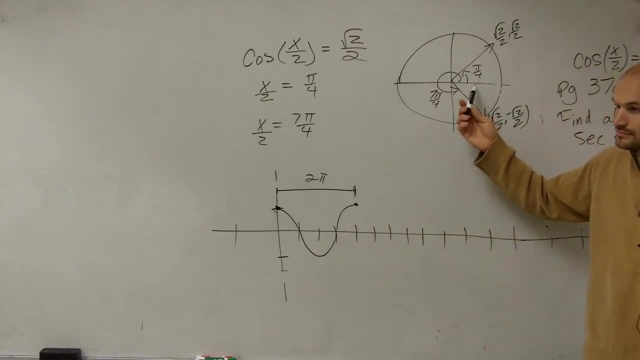 Now we understood, though, that the cosine graph is not just Sorry. the trigonometric functions are not just limited to one revolution. right, We have infinite many revolutions that we can go on. So this graph is going to continue in the positive and negative direction. 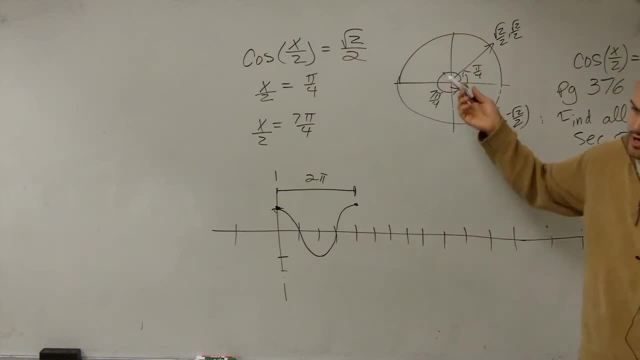 Now we're looking at our answer of when of x equals equals the square root of 2 over 2.. Now, if you kind of look at the decimal version of that, it's going to be less than I'm sorry. yeah, the positive. 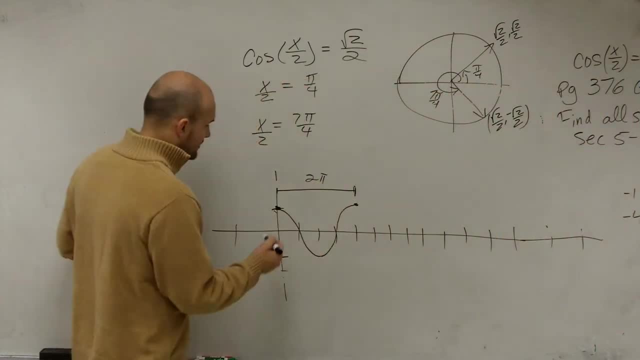 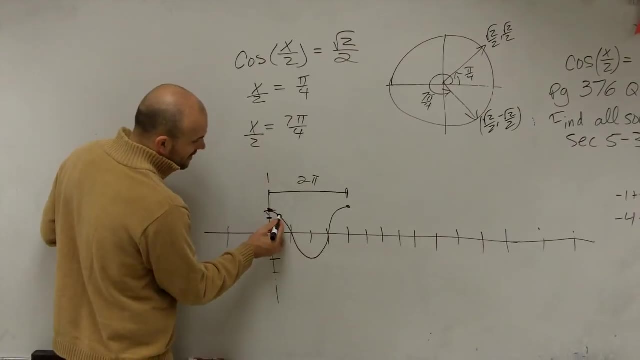 It's going to be less than 1, but greater than 0. And I don't know. let's just pretend the answer's somewhere right around there. All right, So you can see. on the interval of 0 and 2 pi, we have one answer. 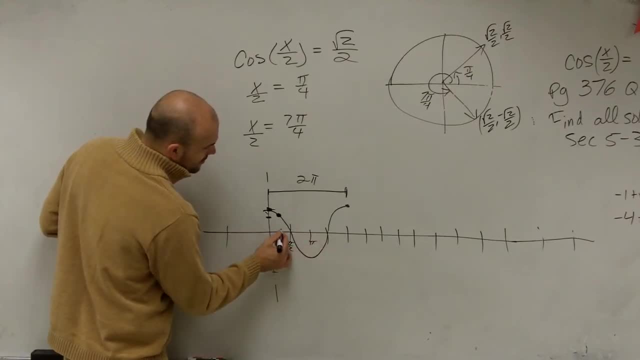 Because if here is pi, here's pi halves, Well then that would be pi fourths. And then our other answer, which would be like right around there, which ends up being: if this is 3, pi over 2,. 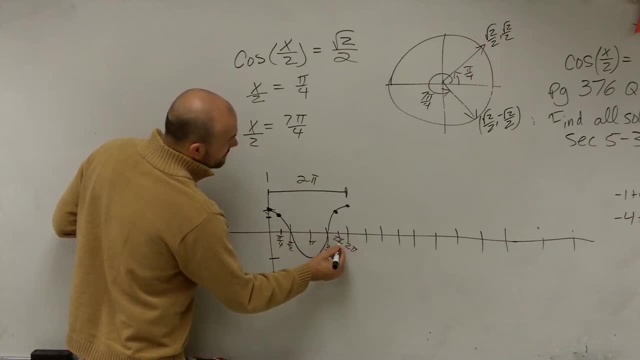 which ends up being: if this is 3 pi over 2,, which ends up being: if this is 3 pi over 2, because this is 2 pi, then that looks like 7 pi, 7 pi over 4.. All right, 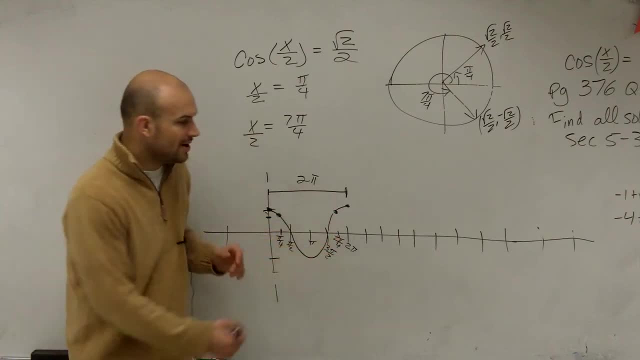 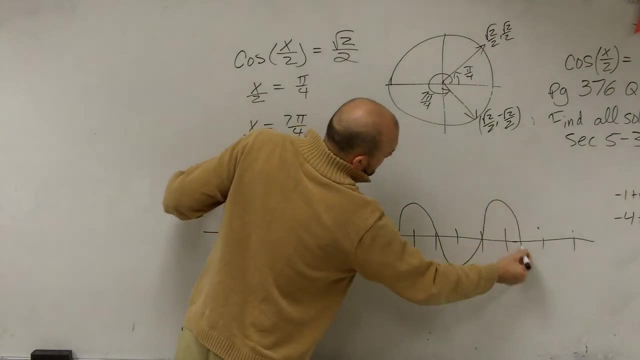 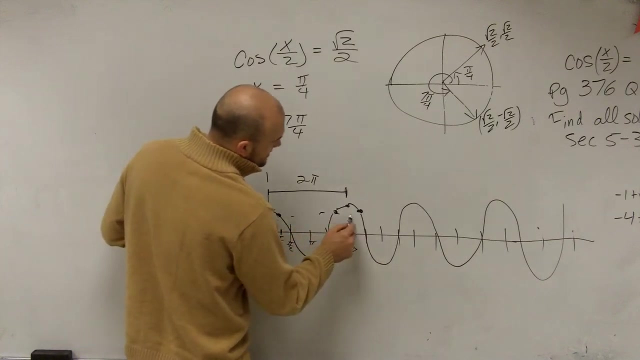 So you guys can see there's two solutions on our graph, right? But notice, ladies and gentlemen, this graph continues, Right, And guess what? There's going to always be this answer on this when our x is equal to square root of 2 over 4.. 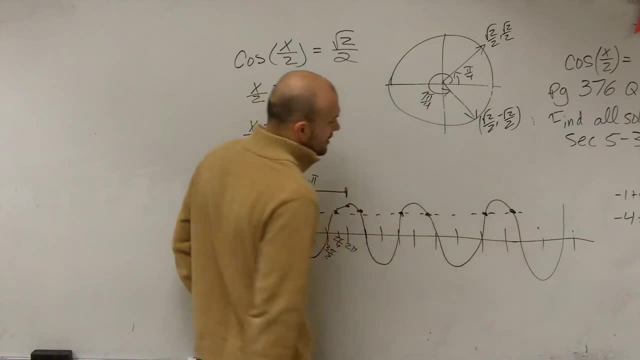 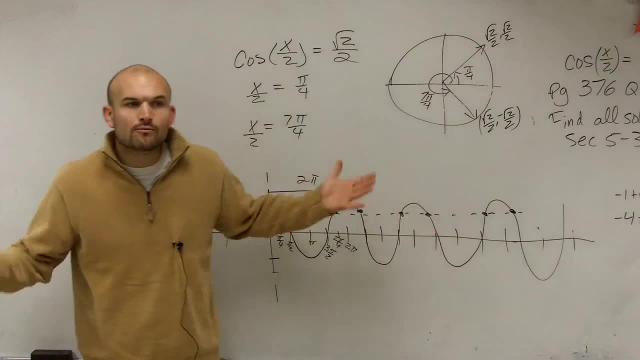 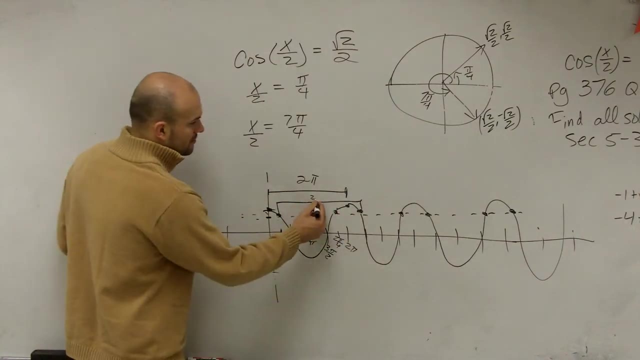 There's infinite many solutions. So how do I represent all of my solutions? Well, I have this solution. To get to the next solution, I have to add what? 2 pi Here to here. 2 pi Here to here. 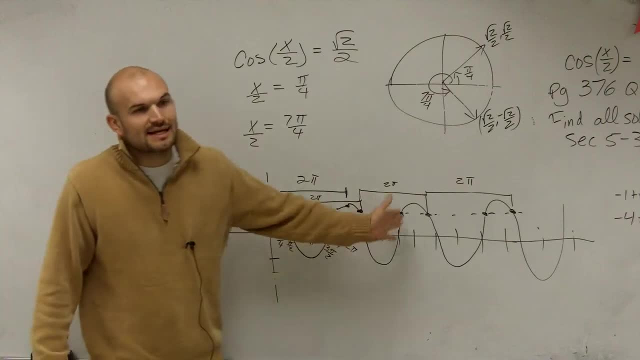 I have to add 2 pi. And how many times can I keep on adding or subtracting 2 pi to always get 2 pi? I have to add 2 pi. How many times can I get my solutions? Infinite, many times. 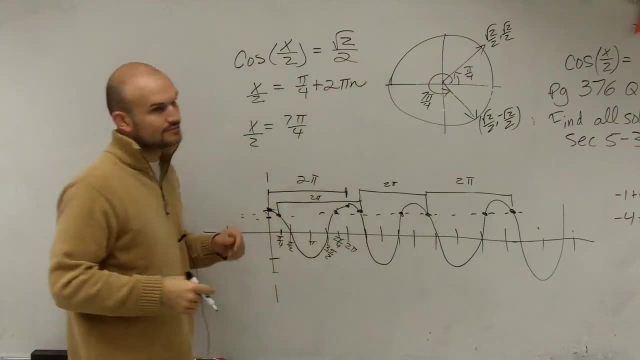 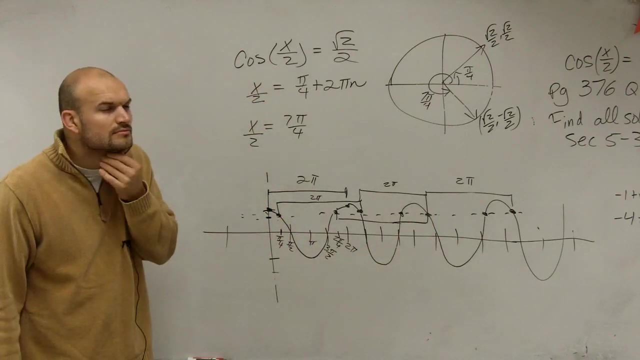 So that's why we're going to write pi over 4 plus 2 pi n. Then the same thing for 7 pi over 4.. To go to 7 pi over 4, to get to the next solution, Should we use 2 pi over 2 to get 2 pi over x. 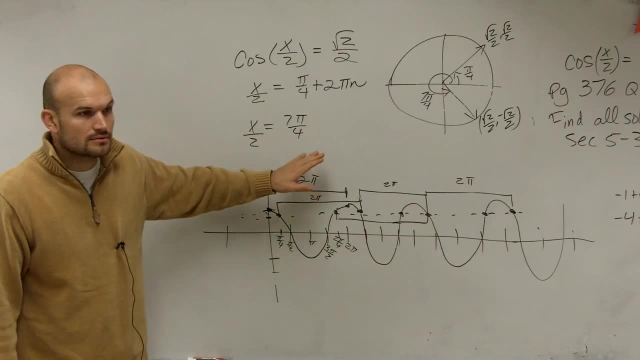 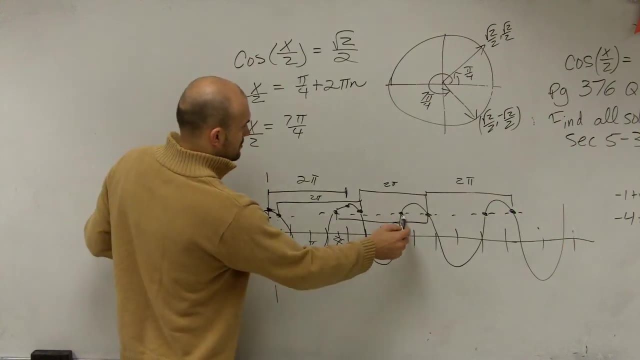 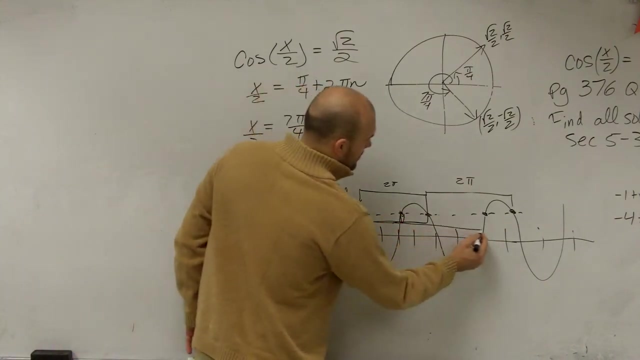 Yeah, I'm going to do that next. Oh, okay, So 2 pi n. And look at my graph. It looks like it's a little rough on its edges, But you can see that each distance for this one to get to the other solution is also going to be. keep on adding 2 pi.